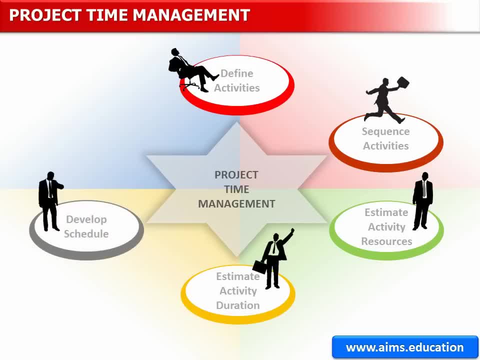 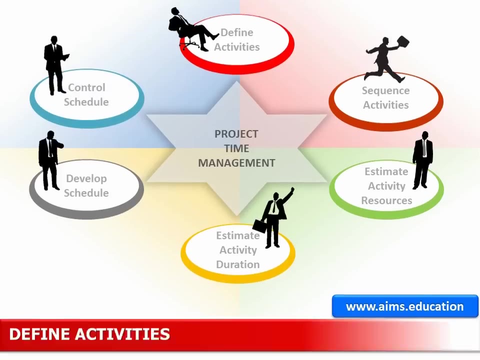 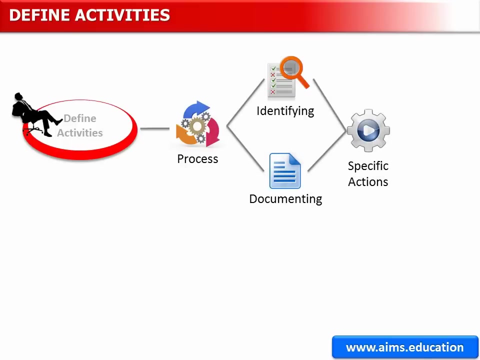 develop schedule. the process of analyzing activity sequences, durations, resource requirements and schedule constraints. and control schedule. the process of monitoring the status of project activities. define activities is the process of identifying and documenting the specific actions to be performed to produce the project deliverables. the key benefit of this process is to break down work packages into activities that 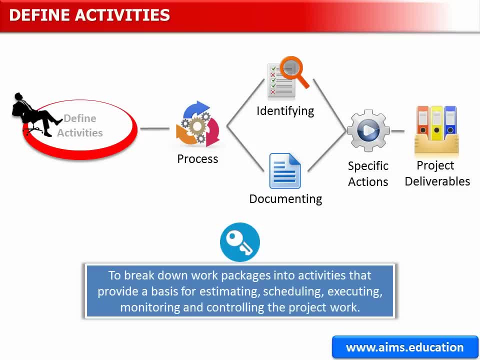 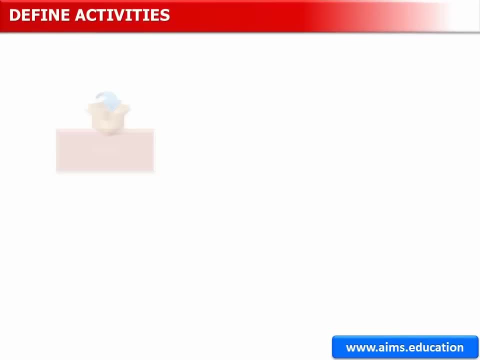 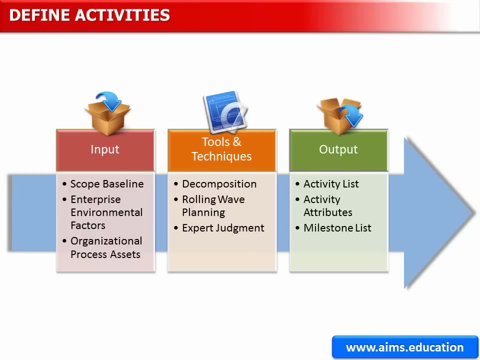 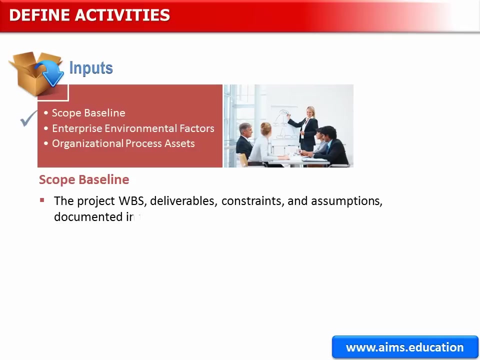 provide a sys for estimating, scheduling, executing, monitoring and controlling the project work. the inputs, tools and techniques and outputs of this process are depicted in this figure: scope baseline. the project WBS deliverables, constraints and assumptions documented in the scope baseline are considered explicitly while defined by the WBS model. 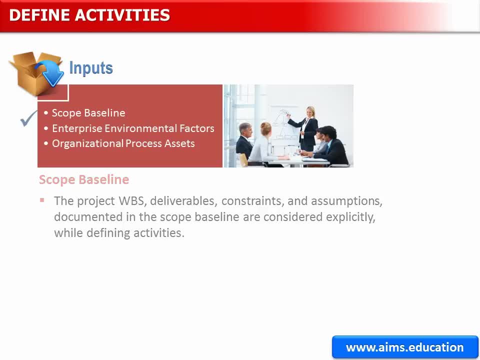 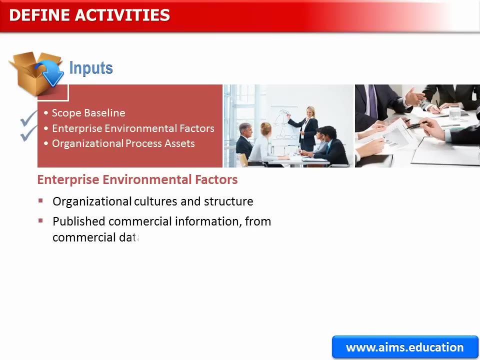 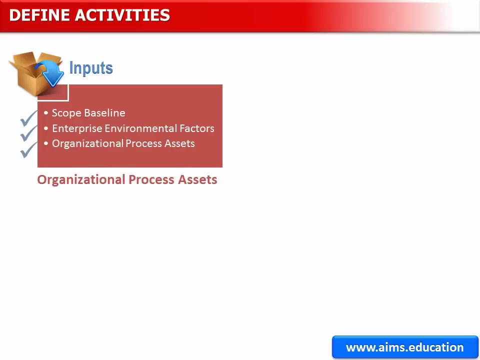 Defining activities Enterprise. environmental factors that influence the define activities process include, but are not limited to, organizational cultures and structure, published commercial information from commercial databases and project management information system. The organizational process assets that can influence the define activities process include: 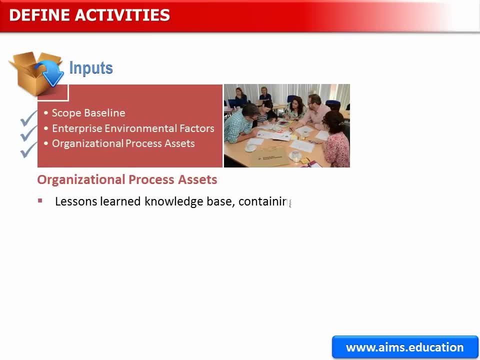 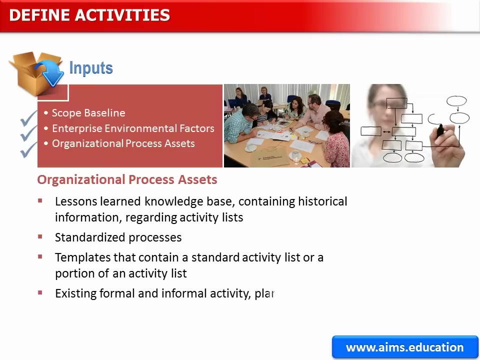 but are not limited to lessons learned. knowledge base containing historical information regarding activity lists used by previous similar projects, Standardized processes, Templates that contain a standard activity list or a portion of an activity list from a previous project, And Formal and informal activity planning related policies, procedures and guidelines. 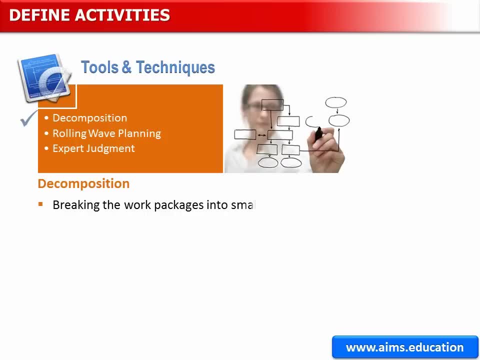 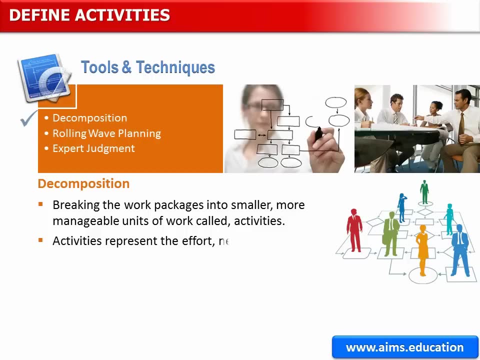 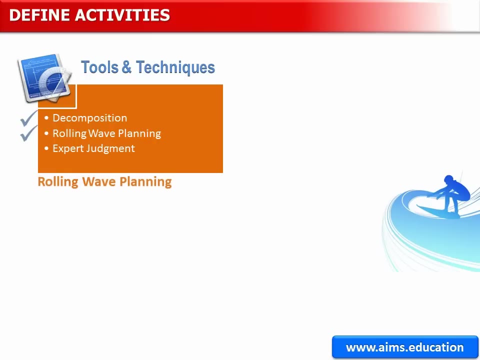 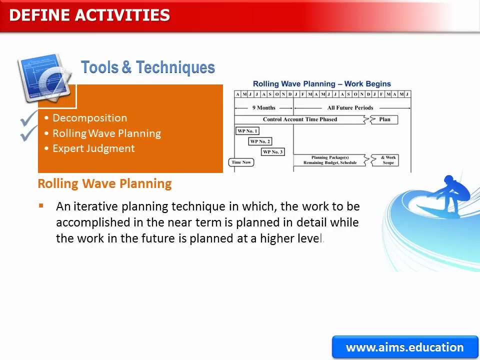 Decomposition involves breaking the work packages into smaller, more manageable units of work called activities. Activities represent the effort needed to complete a work package. Rolling wave planning is an iterative planning technique in which the work to be accomplished in the near term is planned in detail, while the work in the future is planned at a higher. 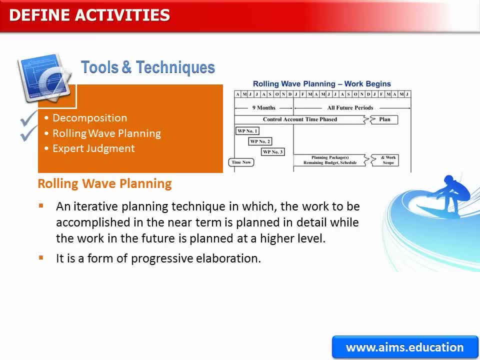 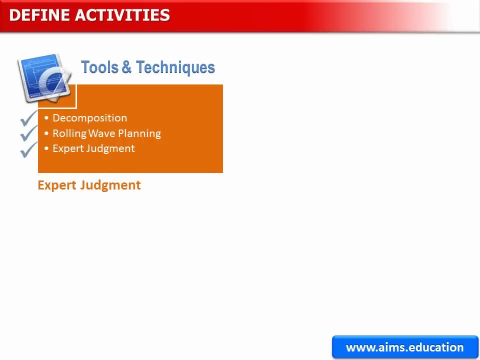 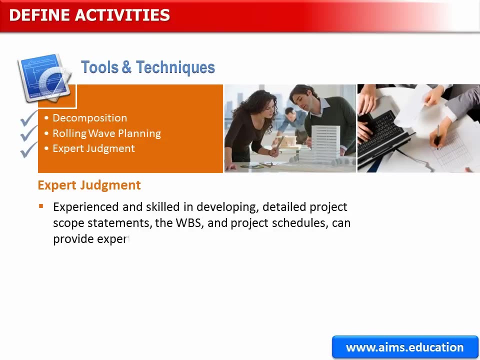 level. It is a form of progressive elaboration. Expert judgment, Project team members or other experts who are experienced and skilled in developing detailed project scope statements, the WBS and project schedules can provide expertise in defining activities. Outputs for define activities. 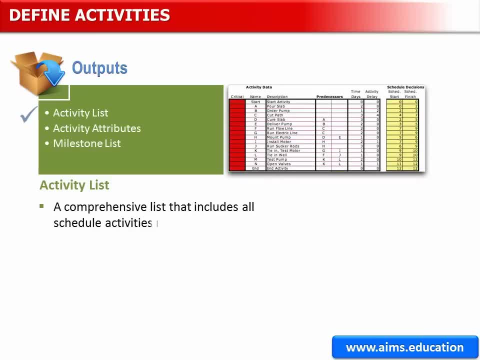 The activity list is a comprehensive list that includes or schedule activities required on the project. The activity list also includes the activity identifier and the scope of work description for each activity in sufficient detail to ensure that project team members understand. 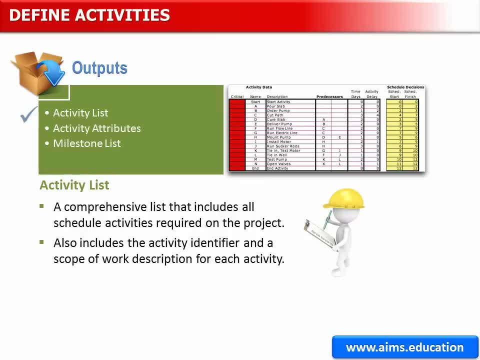 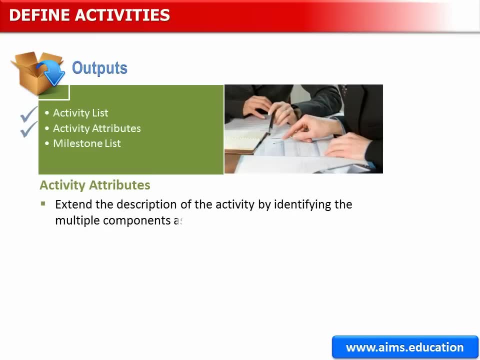 what work is required to be completed. Activity attributes extend the description of the activity by identifying the multiple components associated with each activity. Activity attributes can be used to identify the person responsible For executing the work, geographic area or place where the work has to be performed. 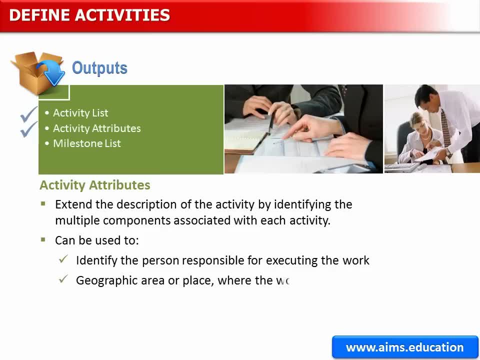 the project calendar the activity is assigned to and activity type. Activity attributes are used for scheduling and to plan tasks and operations By responsible activities. activity attributes can be used to identify the person responsible schedule development and for selecting, ordering and sorting the planned schedule activities. 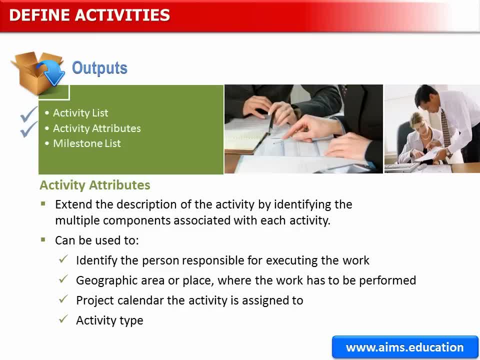 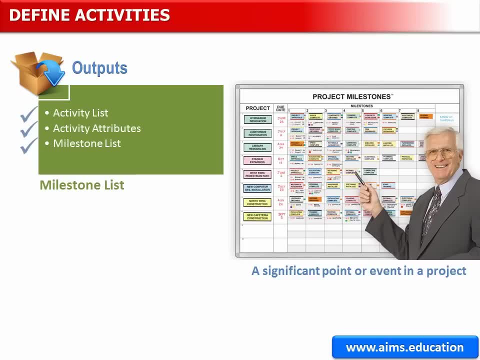 in various ways. within reports, A milestone is a significant point or event in a project. A milestone list is a list identifying all project milestones and indicates whether the milestone is mandatory, such as those required by contract, or optional, such as those based upon historical information. 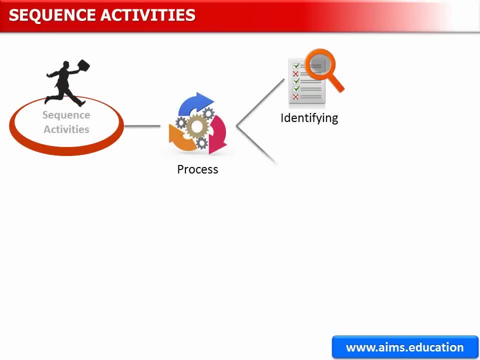 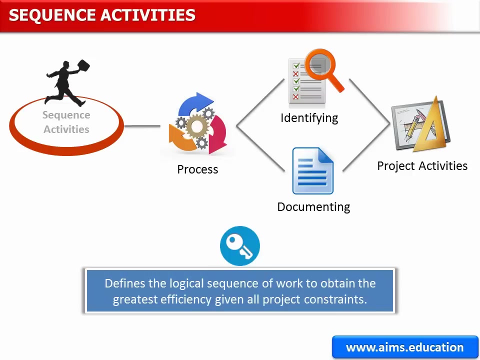 Sequence activities is the process of identifying and documenting relationships among the project activities. The key benefit of this process is that it defines the logical sequence of work to obtain the greatest efficiency given all project constraints: The inputs tools and techniques and the outputs tools. 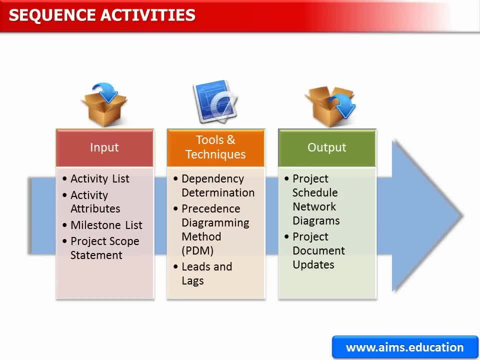 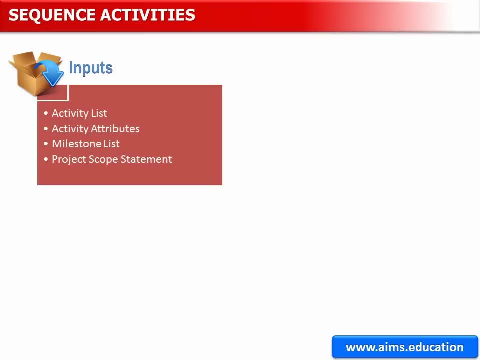 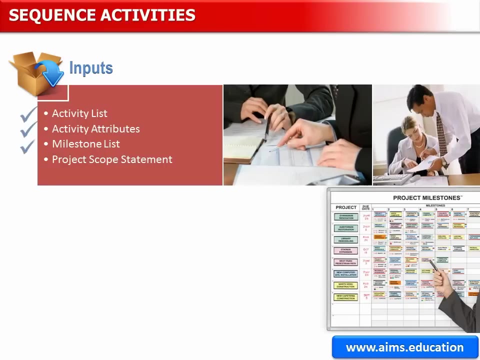 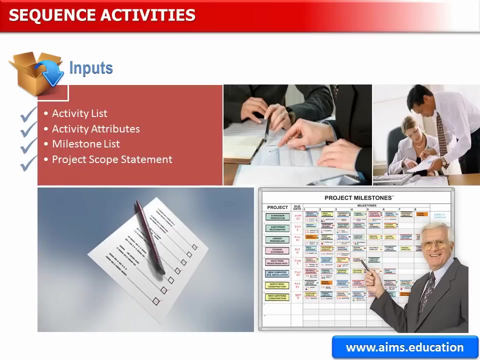 Outputs of this process are depicted in this figure: Inputs for sequence activities. We have already discussed all the inputs to this process. They are activity list, activity attributes, milestone list and project scope statement. Next we will look at several new tools and techniques. 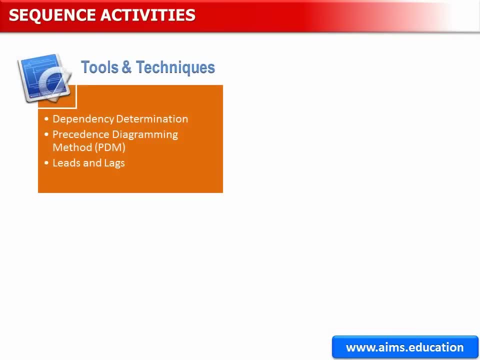 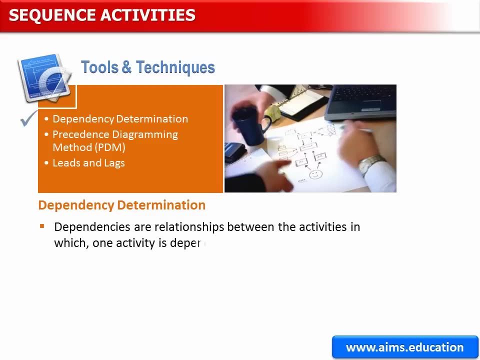 Tools and techniques for sequence activities. Dependencies, Determination. Dependencies are relationships between the activities in which one activity is dependent on another to complete an action, or perhaps an activity is dependent on another to start an action before it can proceed. 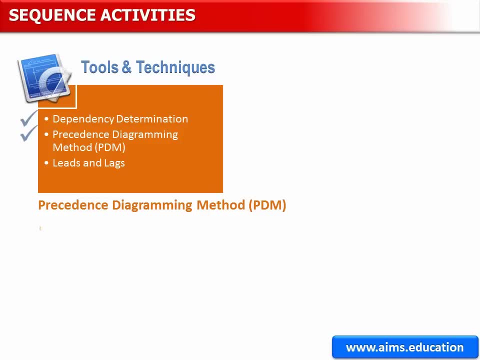 Precedence Diagramming Method: A technique used for constructing a schedule model in which activities are dependent on each other. Activities are represented by nodes and are graphically linked by one or more logical relationships to show the sequence in which the activities are to be performed. 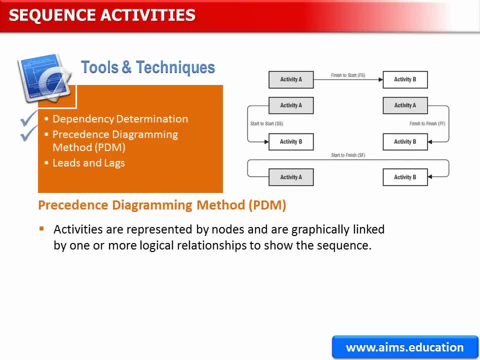 The most common method of arranging the project activities visually. Activities are put in boxes, called nodes, and connected with arrows, called dependencies. Therefore it is known as activity on node. The content of the activity is defined by the activity on node. 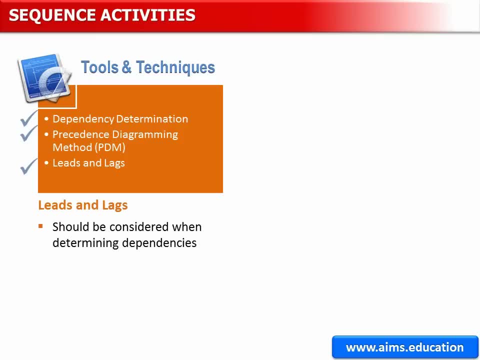 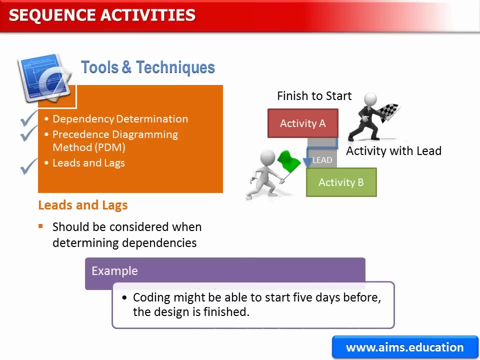 The content covered in this chapter includes Project Time Management, Define Activities, Sequence Activities, Estimate Activity Resources, Estimate Activity Durations, Develop, Schedule And Control Schedule. A lag is a waiting time Inserted in the schedule. A lag is a waiting time. 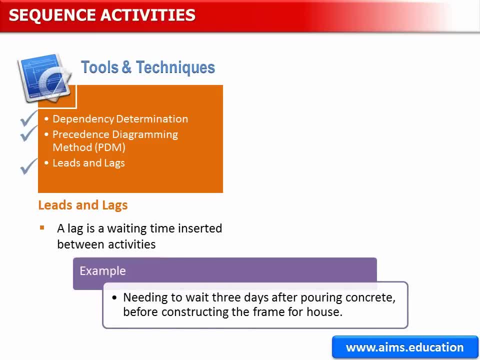 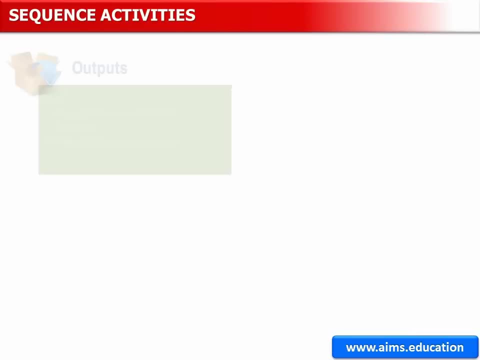 Inserted in the schedule. A lag is a waiting time Inserted between activities, such as needing to wait three days after pouring concrete before constructing the frame for house. Lag time is the delay between the first and second activity. Outputs for Sequence Activities. 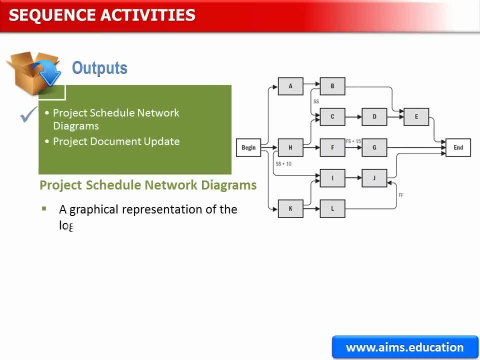 A project schedule network diagram is a graphical representation of the logical relationships, also referred to as dependencies, among the project schedule activities. Figure illustrates a project schedule network diagram. A project schedule network diagram is produced manually or by using project management software. It can include full project details or have one or more summary activities. 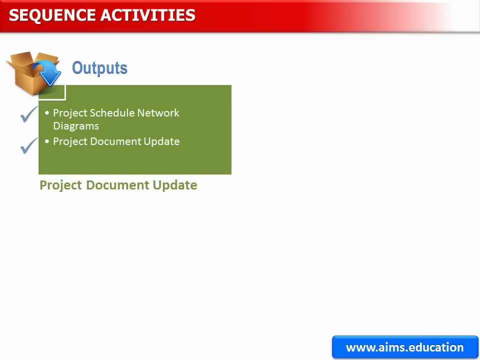 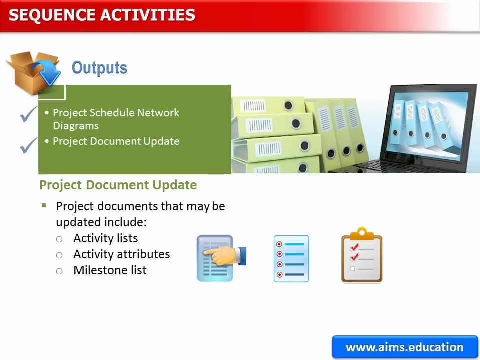 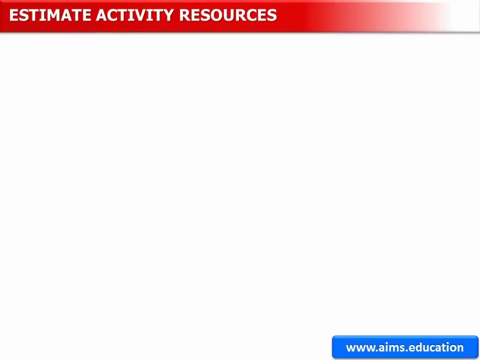 Project documents that may be updated include, but are not limited to, Activity lists, Activity Attributes, Milestone List and Risk Register. Estimate Activity Resources is the process of estimating the type and quantities of material human resources, equipment or supplies required to perform each activity. 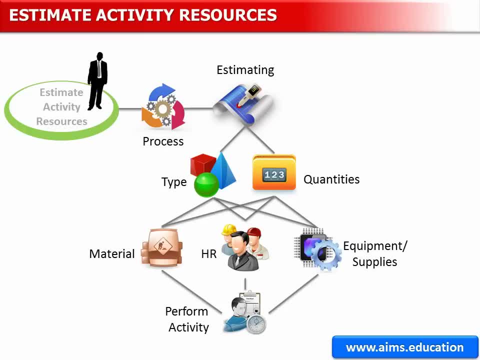 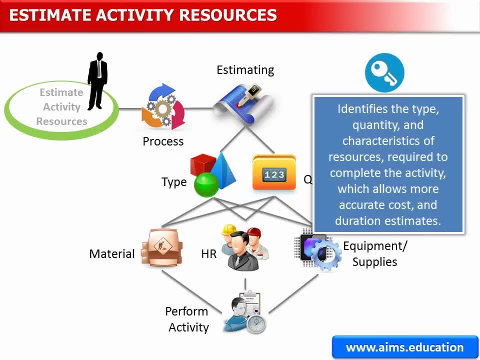 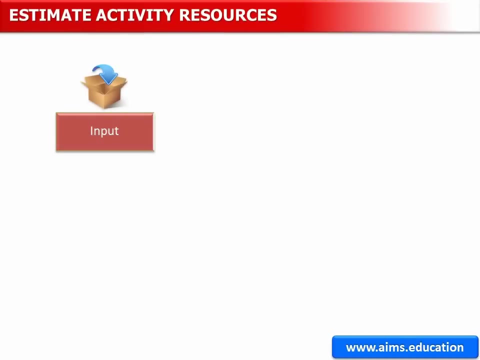 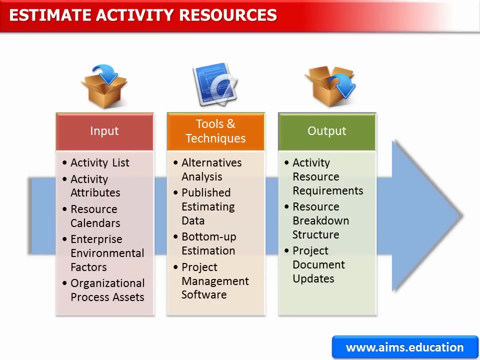 The key benefit of this process is that it identifies the type, quantity and characteristics of resources required to complete the activity, which allows more accurate cost and duration estimates. The inputs, tools and techniques and outputs of this process are depicted in this figure. 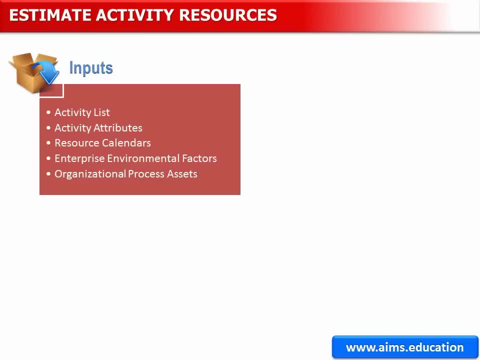 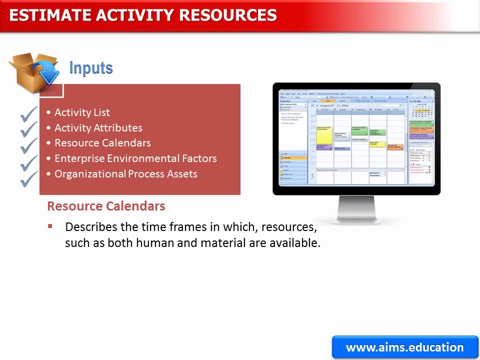 Inputs for Estimate Activity Resources. This process has several inputs, most of which you already know, such as Activity List, Activity Attributes, Enterprise Environmental Factors and Organizational Process Assets. Only input we have not discussed before is Resource Calendars. The Resource Calendars describes the time frames in which resources, such as both human and material, are available. 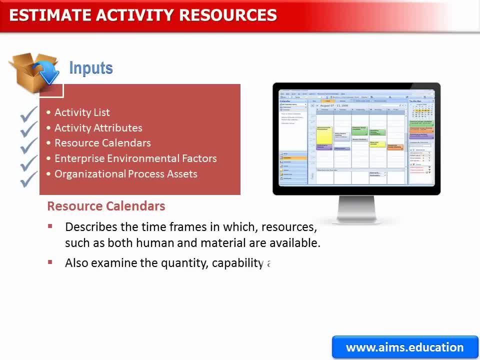 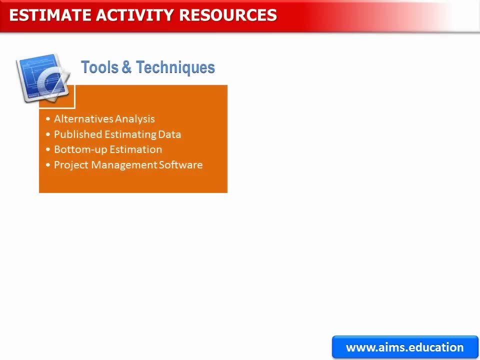 Resource Calendars- Resource Calendars. Resource Calendars also examine the quantity, capability and availability of equipment and material resources that have a potential to impact the project schedule. Tools and Techniques for Estimate Activity Resources. Alternative Analysis: Many schedule activities have alternative methods of accomplishment. 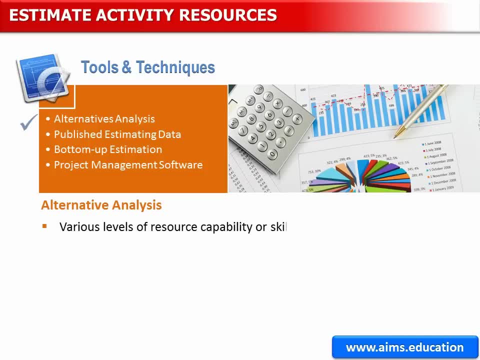 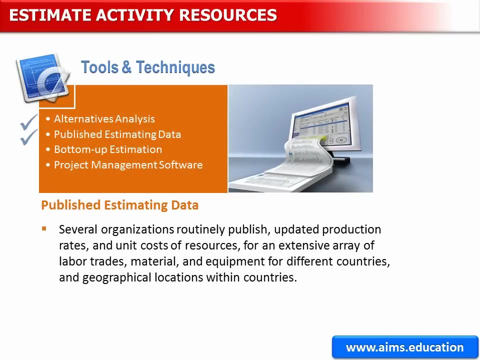 They include using various levels of resource, capabilities or skills, different size or type of machines, different tools- that is, hand versus automated- and make rent or buy decisions regarding the resource. Published Estimating Data: Several organizations routinely publish updated production rates and unit costs of resources. 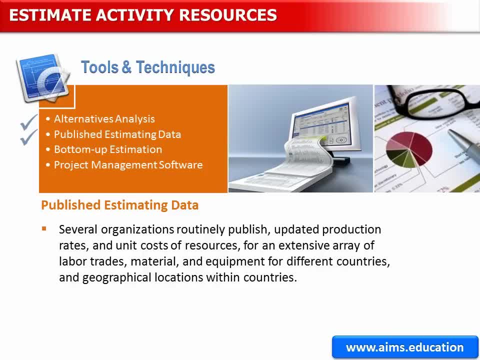 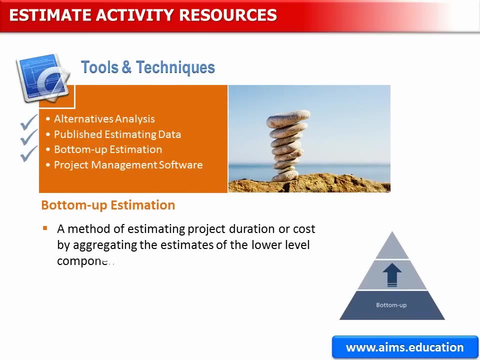 for an extensive array of labor, trades, material and equipment for different countries and geographical locations within countries. Bottom-up Estimating. Bottom-up Estimating is a method of estimating project duration or cost by aggregating the estimates of the lower level components of the WBS. 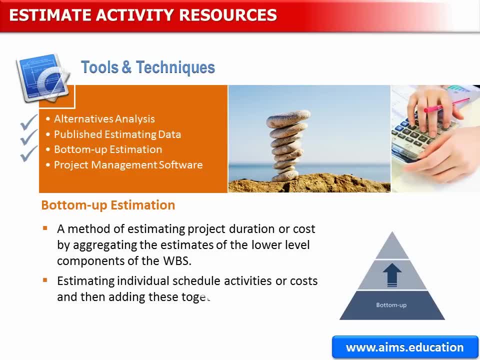 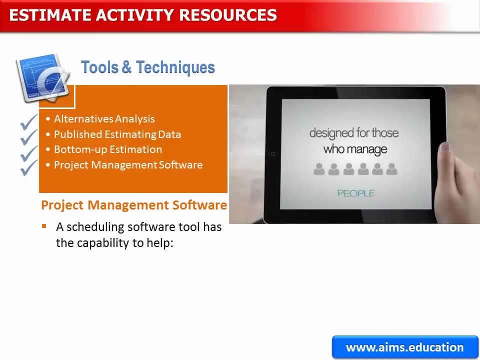 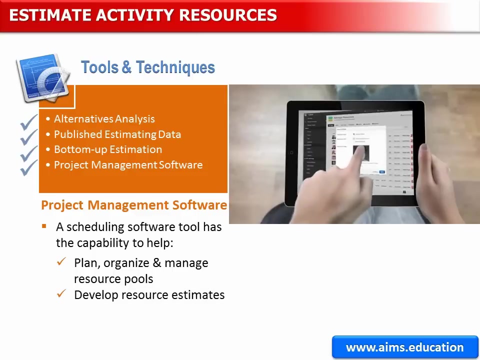 estimating individual schedule activities or costs and then adding these together to come up with a total estimate for the work package. Project management software, such as a scheduling software tool, has the capability to help plan, organize and manage resource pools and develop resource estimates. 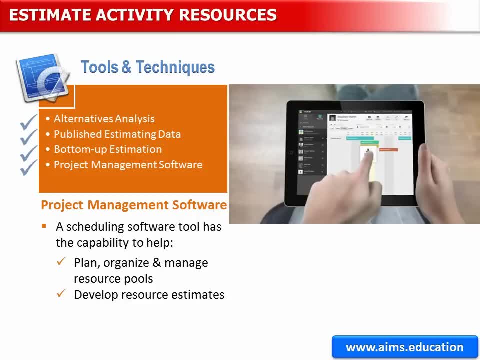 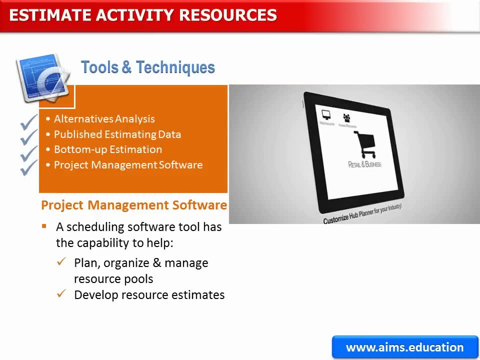 Depending on the sophistication of the software, resource breakdown structures, resource availability, resource rates and various resource calendars can be defined to assist in optimizing resource utilization. Bottom-up Estimating: Bottom-up Estimating is a tool that allows we to analyze documentation and format. 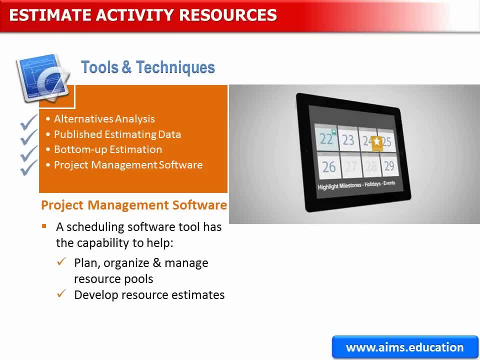 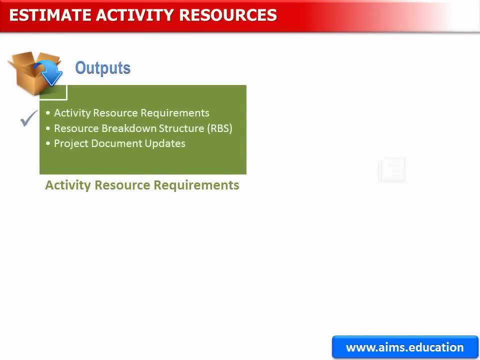 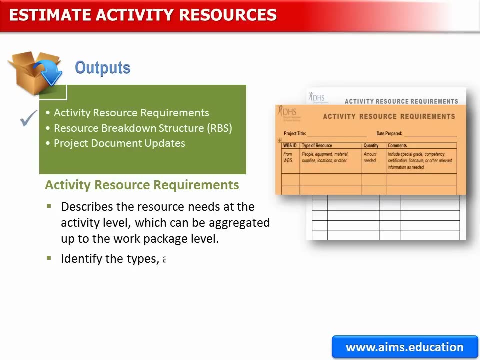 historical NAV placeholder objectives and viendo effect. updates of Ying rule's standards and families. explanation of cell property criteria. Outputs for estimate activity resources. The activity resource requirements document describes the resource needs at the activity level which can be aggregated up to the work package level. 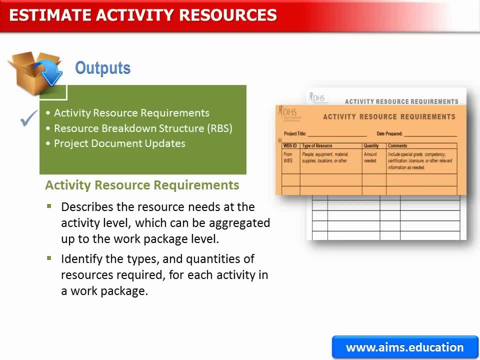 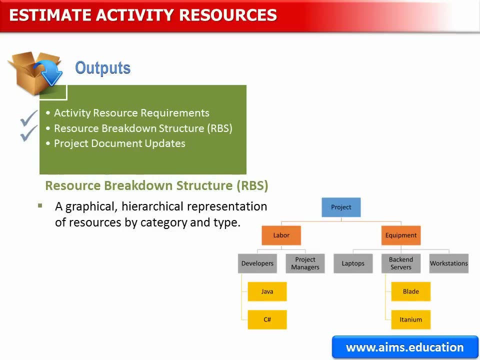 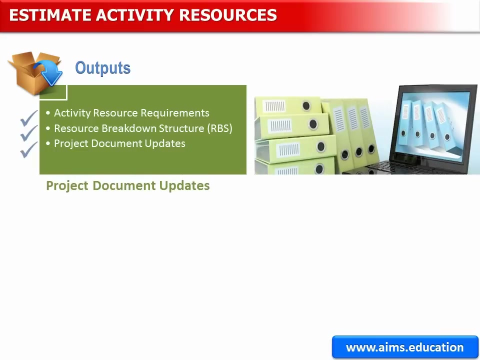 Activity resource requirements. identify the types and quantities of resources required for each activity in a work package. The resource breakdown structure is a hierarchical representation of resources by category and type. Examples of resource categories include labor, material equipment and supplies. Project documents that may be updated include, but are not limited to, activity list, activity attributes and resource calendars. 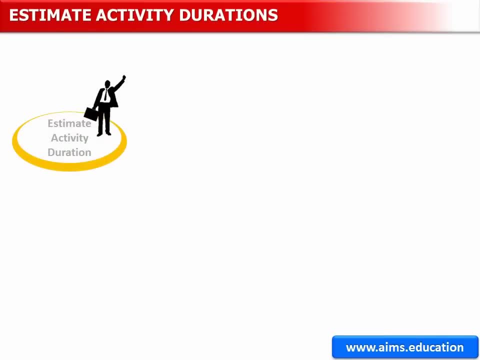 Estimate activity durations is the process of estimating the number of work periods needed to complete individual activities with estimated resources. The activity duration is the process of estimating the number of work periods needed to complete individual activities with estimated resources. Work periods are usually expressed in hours or days. 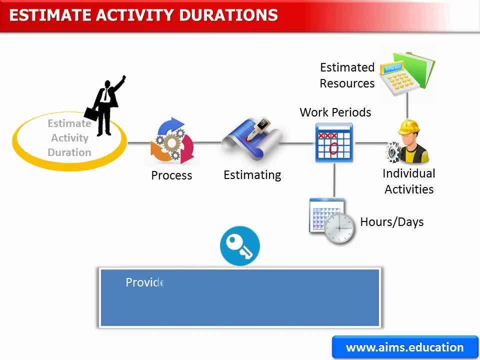 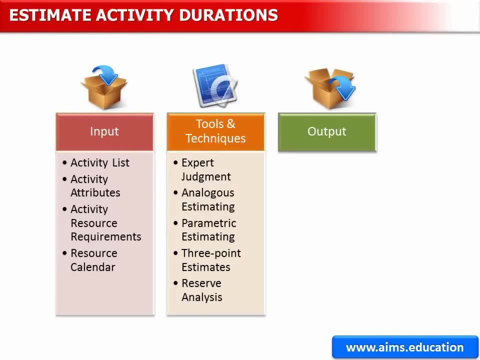 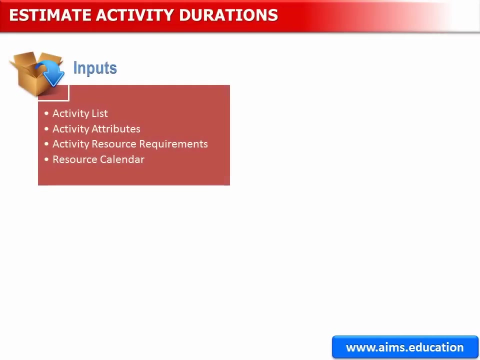 The key benefit of this process is that it provides the amount of time each activity will take to complete, which is a major input into the develop schedule process. The inputs, tools and techniques and outputs of this process are depicted in this figure. Inputs for estimate activity durations. 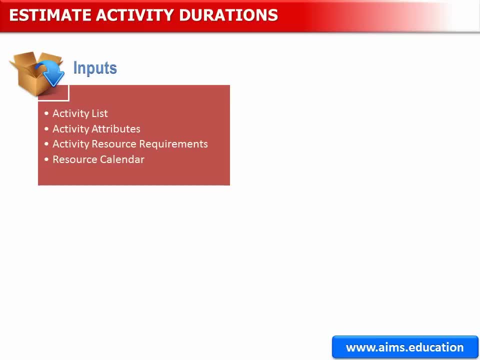 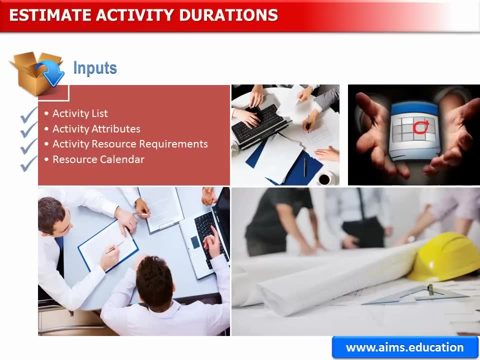 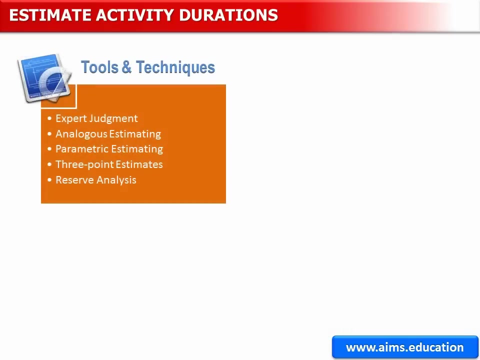 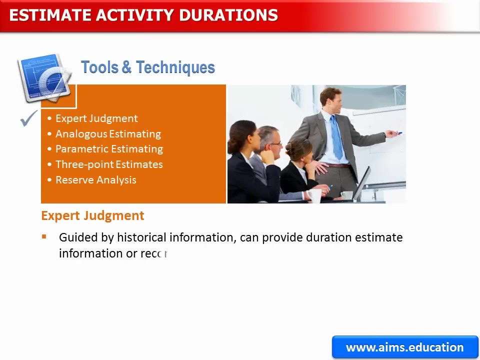 Inputs for estimate activity durations. The inputs to this process include activity list, activity attributes, activity resource requirements and resource calendars, which have already discussed Tools and techniques for estimate activity durations. Expert judgment guided by historical information can provide duracious estimate information or recommended maximum activity durations. 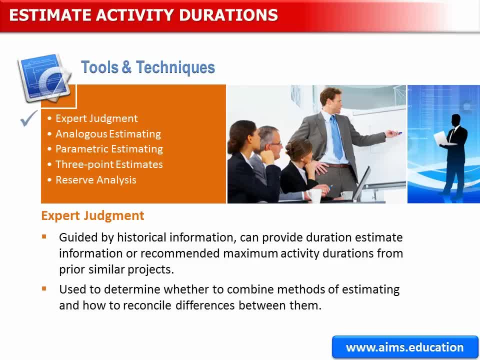 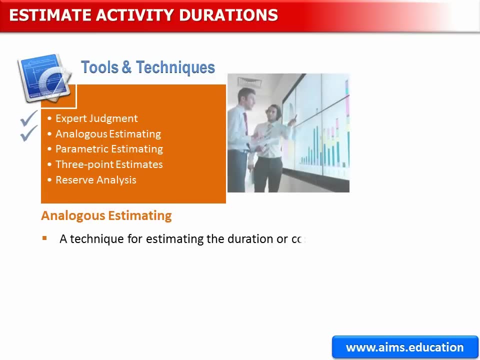 from prior similar projects. Expert judgment can also be used to determine whether to combine methods of estimating and how to reconcile differences between them. Analogous estimating is a technique for estimating the duration or cost of an activity or a project using historical data from a similar activity or project. 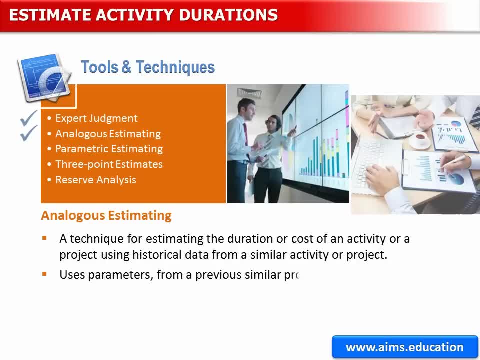 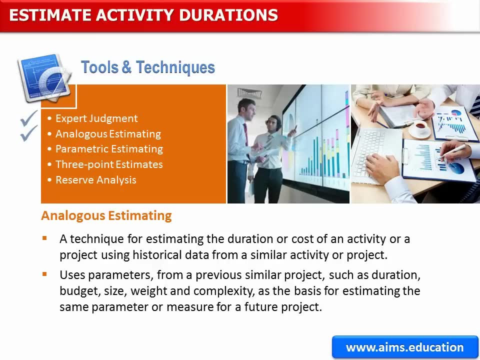 Analogous estimating uses parameters from a project to a project. Analogous estimating uses parameters from a project to a project. Analogous estimating uses parameters from a previous similar project, such as duration, budget size, weight and complexity, as the basis for estimating the same parameter or measure for a future project. 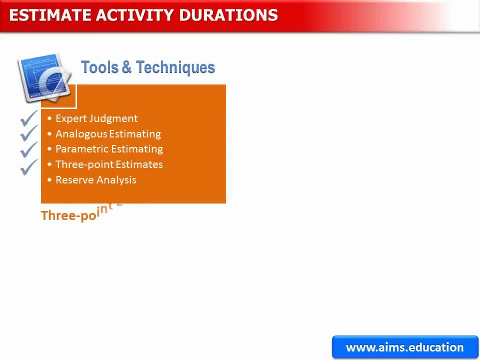 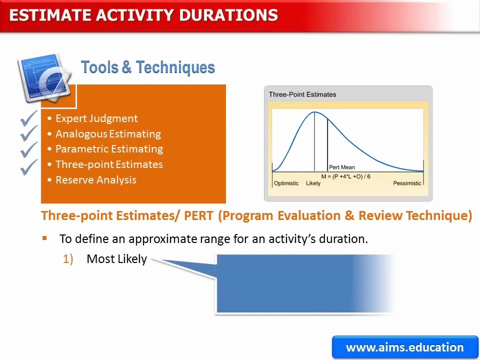 3-point estimates, or PERT, is the acronym for Program Evaluation and Review Technique. PERT uses three estimates to define an approximate range for an activity's duration. Prior: These are estimations for final execution of material-based estimates for the involved target type. 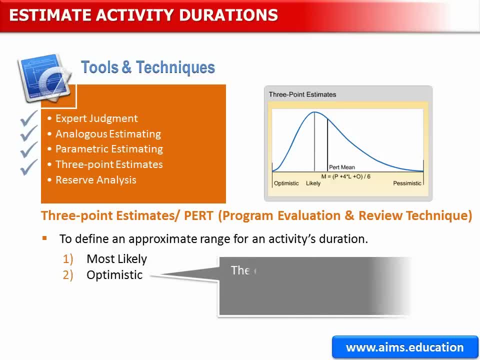 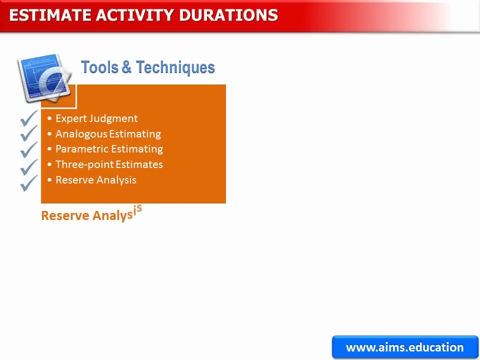 Monitoring Pred Jeremiah Guarantee Resolution: Undo Mobile. Mao Hu C Reserve analysis. Duration estimates may include contingency reserves, sometimes referred to as time reserves, or buffers into the project schedule to account for schedule uncertainty. There are two types of reserves: Contingency reserve and management reserve. 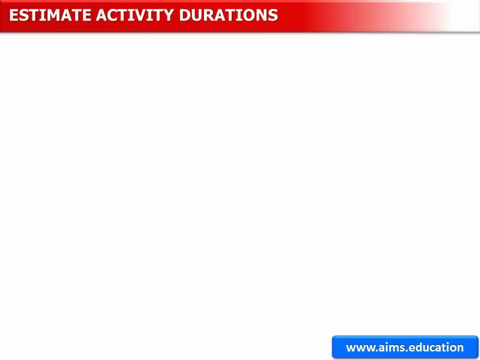 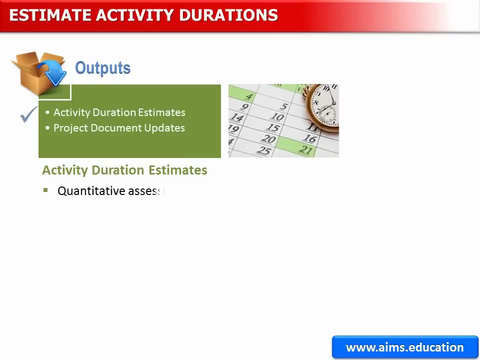 Outputs for estimate activity durations. Activity duration estimates are quantitative assessments of the likely number of time periods that are required to complete an activity. Duration estimates do not include any lags. Project documents that may be updated include, but are not limited to, activity attributes. 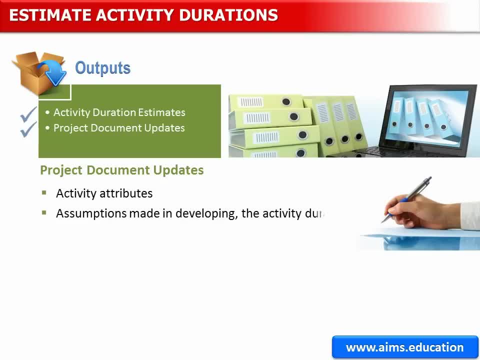 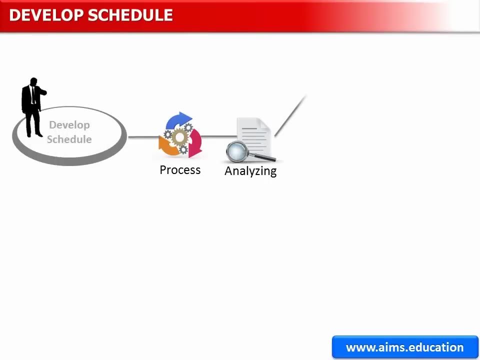 And assumptions made in developing the activity duration estimate, such as skill levels and availability, as well as a basis of estimates for durations. Develop schedule is the process of analyzing activity sequences, durations, resource requirements and schedule constraints to create the project schedule model. 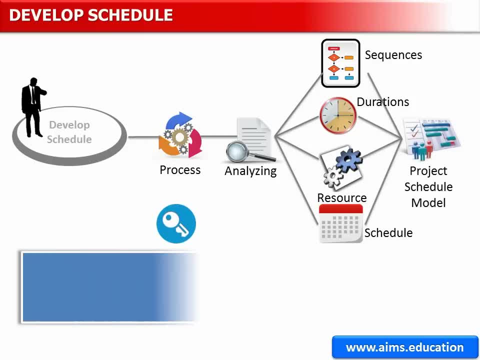 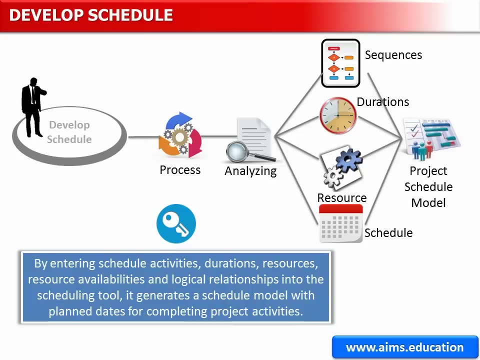 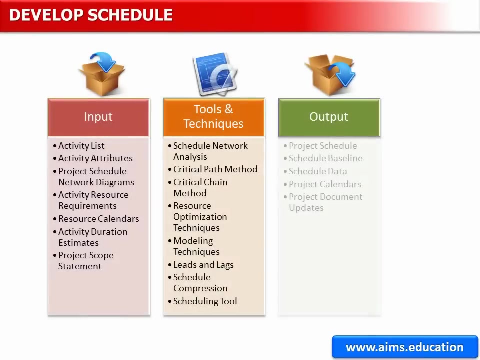 The key benefit of this process is that, by entering schedule, activities, durations, resources, resource availabilities and logical relationships into the scheduling tool, it generates a schedule model with planned dates for completing project activities. The inputs, tools and techniques and outputs of this process are depicted in this figure. 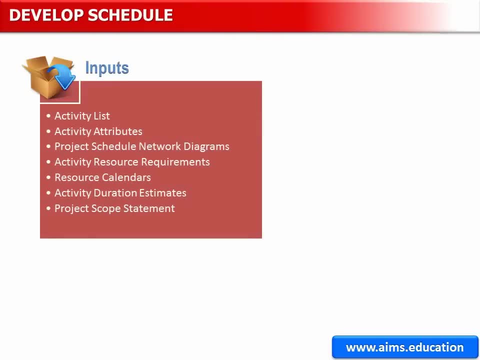 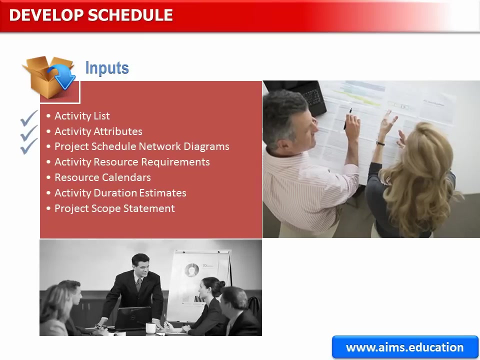 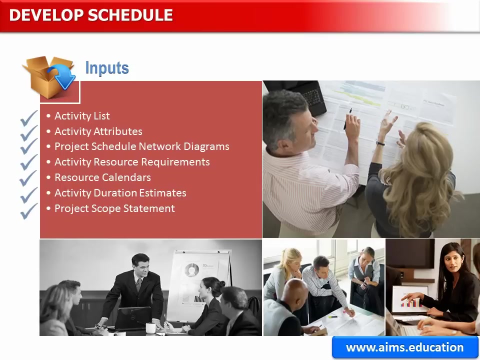 Inputs for develop schedule. It has several inputs- A lot of them have been discussed, which are outputs from other processes. The inputs are as follows: Activity list, Activity attributes, Project schedule, network diagrams, Activity resource requirements, Resource calendars, Activity duration estimates And project scope statement. 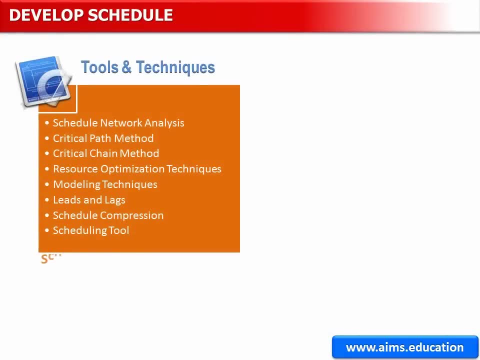 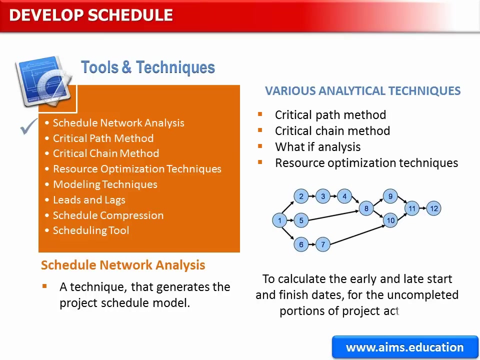 Tools and techniques for develop schedule Schedule. network analysis is a technique that generates the project schedule model. It employs various analytical techniques such as critical path method, critical chain method, Watt of analysis and resource optimization techniques to calculate the early and late start and finish dates for the uncompleted portions of project activities. 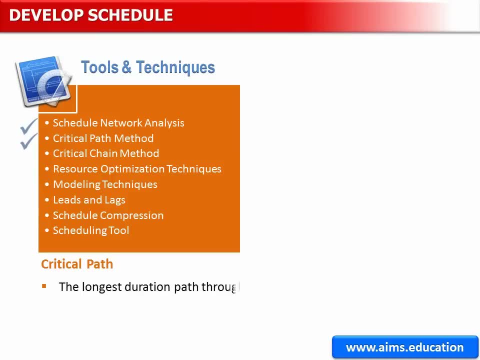 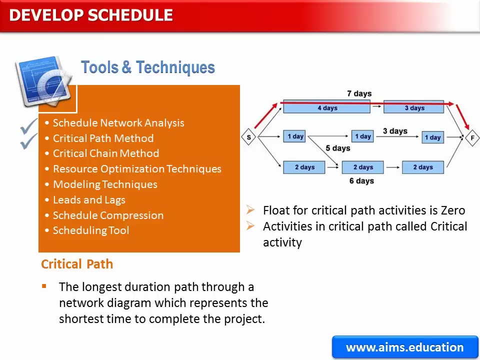 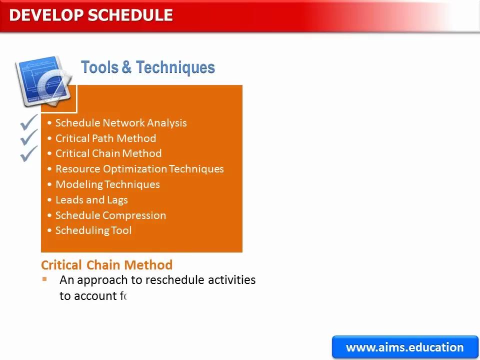 Critical path is the longest duration path through a network diagram which represents the shortest time to complete the project. Float for critical path activities is zero Activities in critical path, called critical activity. Critical chain method is an approach to reach dual activities to account for the limited resources. 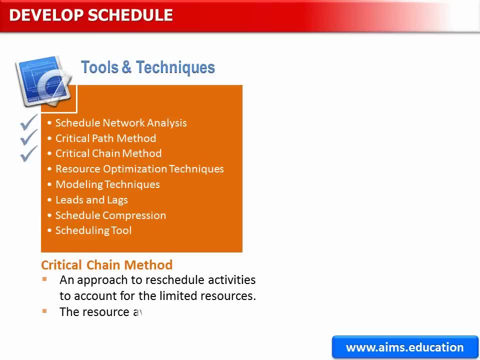 After the schedule is constructed, the project is completed. The resource availability is entered to produce a modified critical path. The resource constrained critical path is known as the critical chain. In this figure, path from start to end through C, D, E and F is the critical chain. 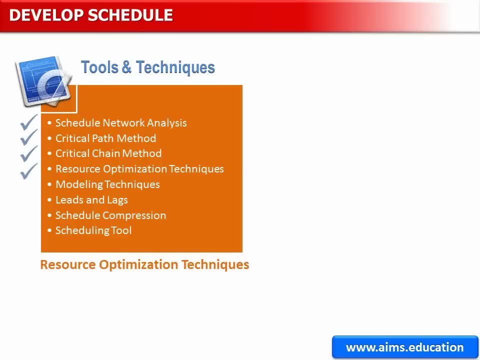 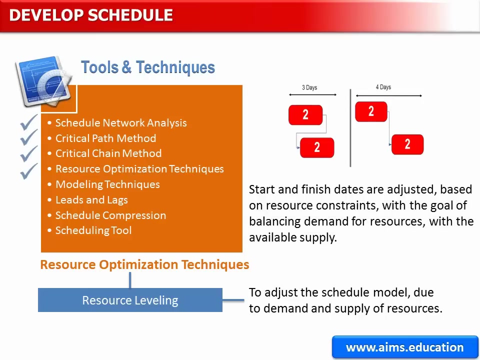 Resource optimization techniques. Examples of resource optimization techniques is resource optimization- Resource leveling- that can be used to adjust the schedule model due to demand and supply of resources. Resource leveling is a technique in which start and finish dates are adjusted based on resource constraints, with the goal of balancing demand for resources with the available supply. 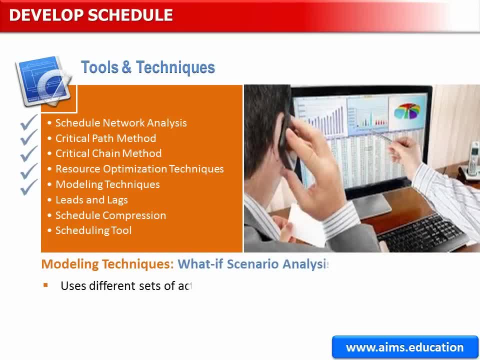 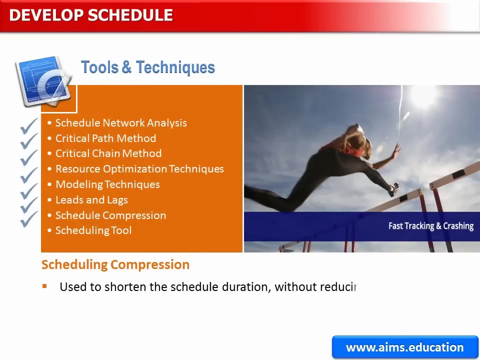 What if scenario analysis uses different sets of activity assumptions to produce multiple project durations? For example, what would happen if a major deliverable was delayed or the weather prevents you from completing a deliverable on time? Schedule compression techniques are used to shorten the schedule duration without reducing the project scope, in order to meet schedule constraints, imposed dates or other schedule objectives. 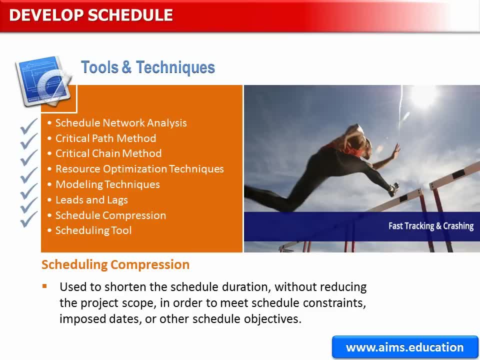 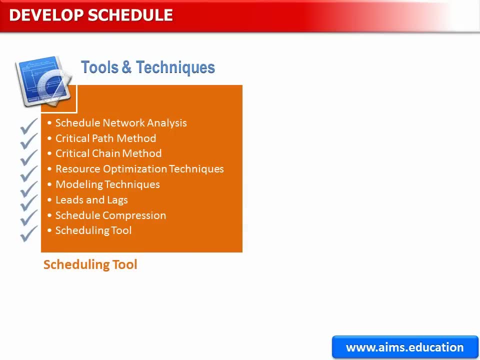 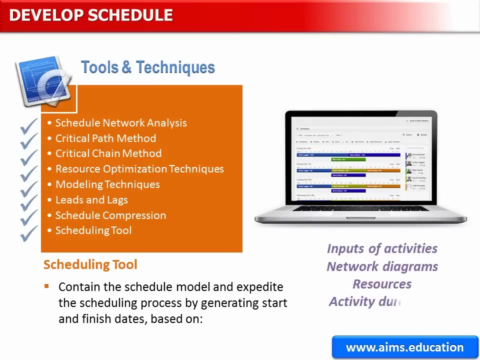 Schedule compression techniques include crashing And fast tracking. Automated scheduling tools contain the schedule model and expedite the scheduling process by generating start and finish dates based on the inputs of activities, network diagrams, resources and activity durations using schedule network analysis. 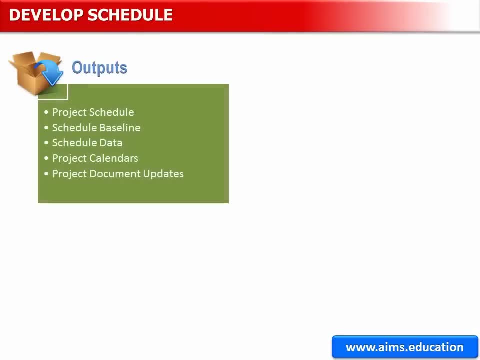 Outputs for develop schedule. The project schedule is an output of a schedule model that presents linked activities with planned dates, durations, milestones and resources. A project schedule model can be presented in tabular form. it is more often presented graphically, which are classified as: 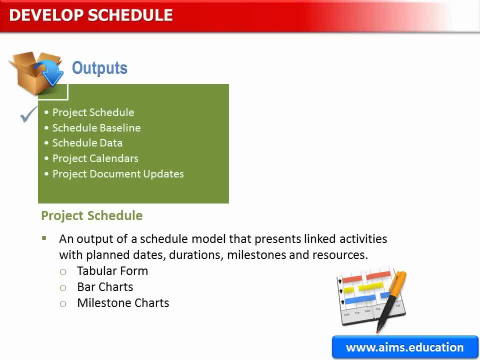 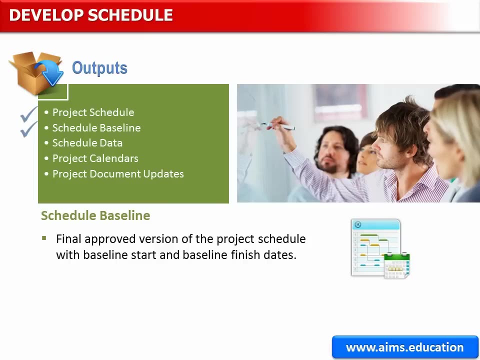 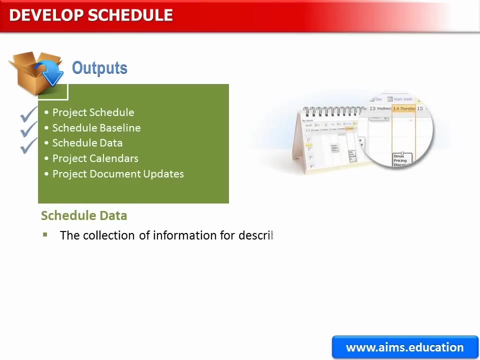 Bar charts, Milestone charts And project schedule network diagrams. A schedule baseline is the final approved version of the project schedule with baseline start and baseline finish dates. The schedule data for the project schedule model is the collection of information for describing and controlling the schedule. 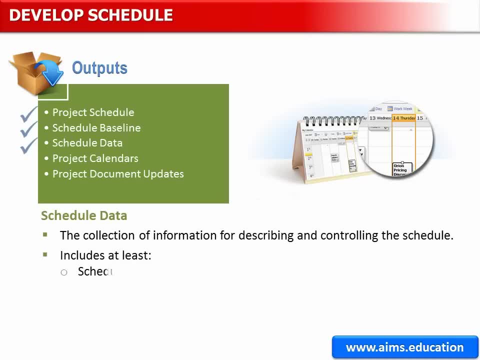 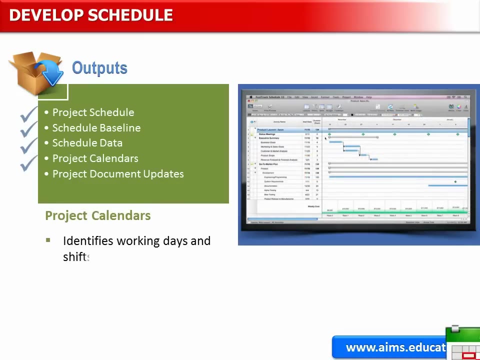 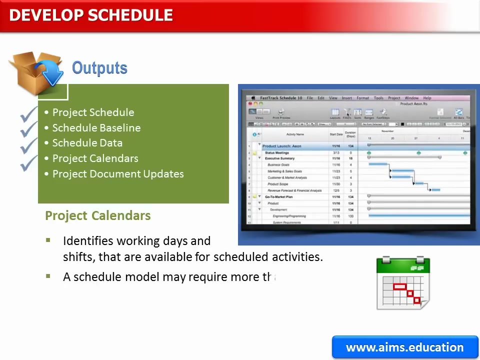 The schedule data includes at least the schedule milestones, schedule activities, activity attributes and documentation of all identified assumptions. A project calendar identifies working days and shifts that are available for scheduled activities. A schedule model may require more than one project calendar to allow for different work periods for some activities. to calculate the project schedule, 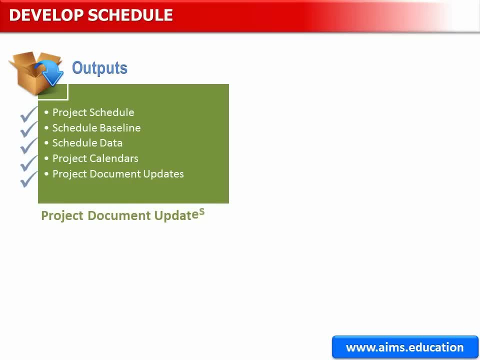 Project documents that may be updated include, but are not limited to, Activity resource requirements. If the resource leveling analysis changes the project resource requirements, then the project resource requirements are updated. Activity attributes are updated to include any revised resource requirements and any other revisions. 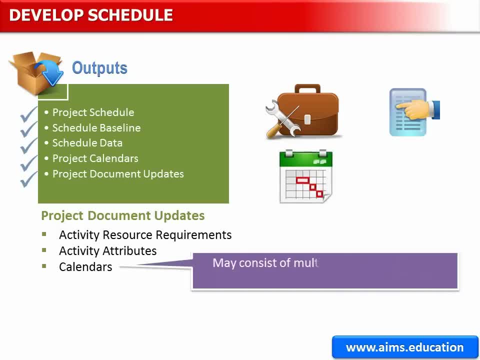 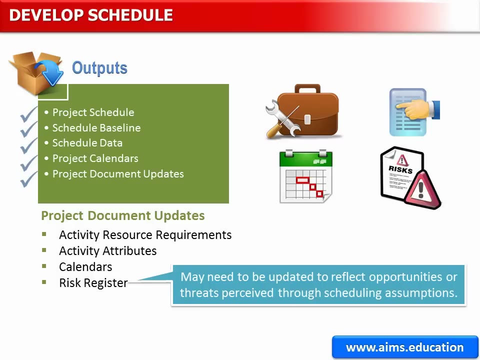 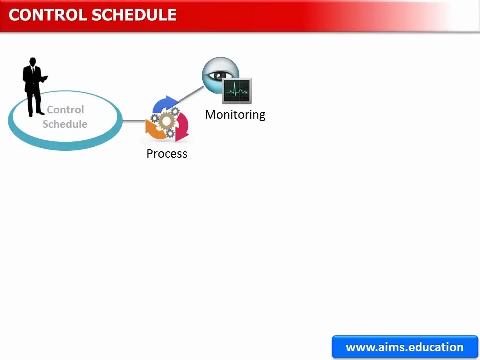 The calendar for each project may consist of multiple calendars: project calendars, individual resources. The risk register may need to be updated to reflect opportunities or threats perceived through scheduling assumptions. Control schedule is the process of monitoring the status of project activities to update project progress and manage changes to the schedule baseline to achieve the plan. 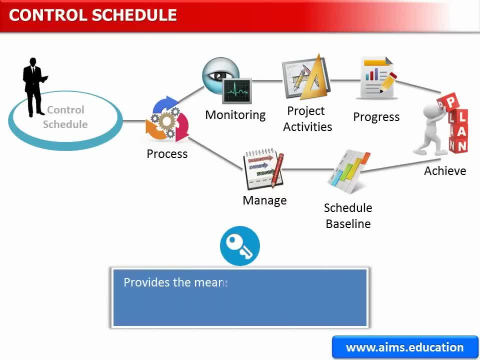 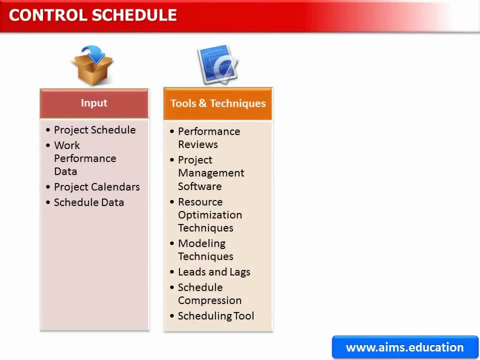 The key benefit of this process is that it provides the means to recognize data, It provides deviation from the plan and take corrective and preventive actions and thus minimize risk. The inputs, tools and techniques and outputs of this process are depicted in this figure. 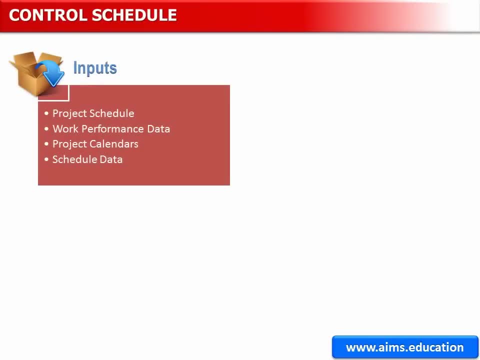 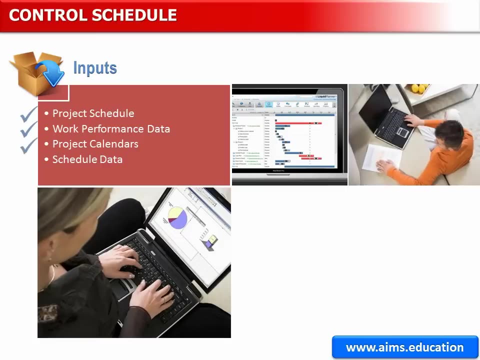 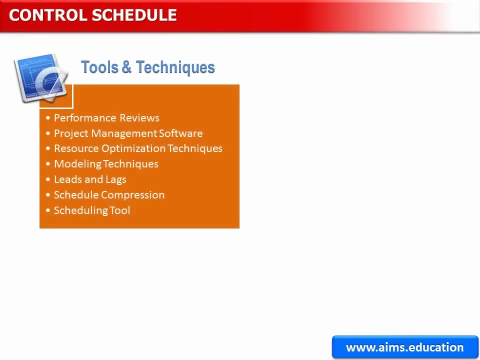 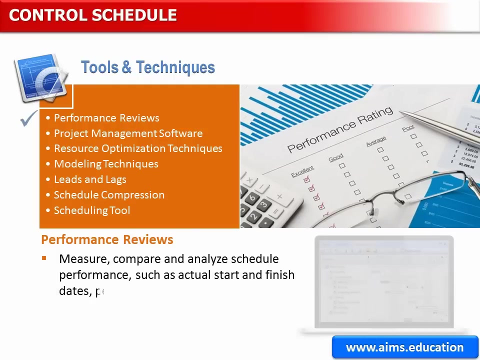 Inputs for control schedule. We have already discussed all the inputs to this process. They are: project schedule, work performance data, project calendars and schedule data. Tools and techniques for control schedule. Performance reviews, measure, compare and analyze schedule performance, such as actual start and finish dates, percent complete and remaining duration for work in progress. 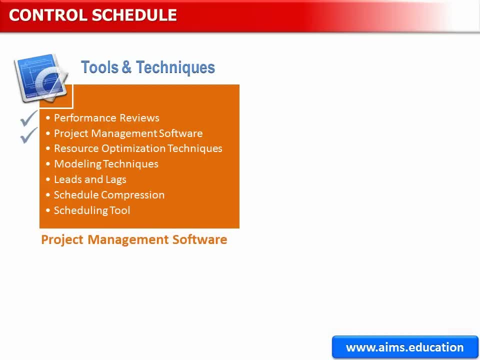 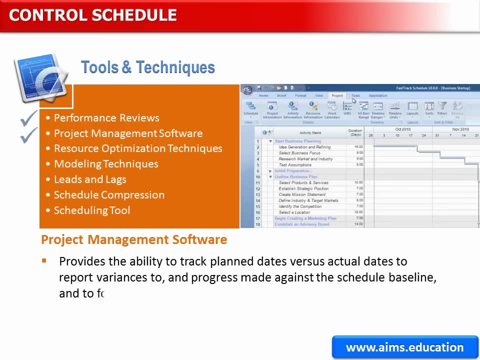 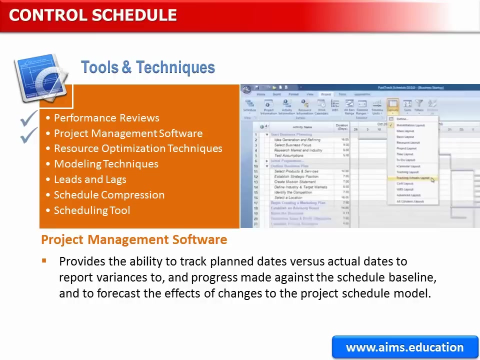 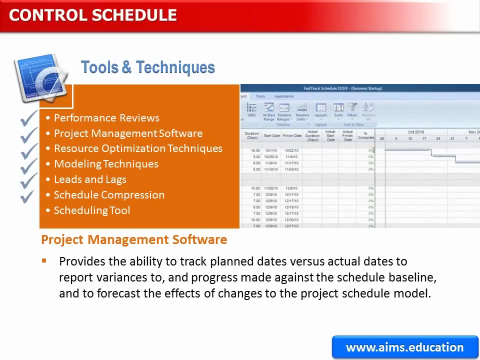 Project management software for scheduling provides the ability to track planned dates versus actual dates, to report variances to and progress made against the schedule baseline and to forecast the effects of changes to the project schedule. model, Resource optimization techniques, modeling techniques, leads and lags, schedule compression and scheduling tool have been discussed in other processes. 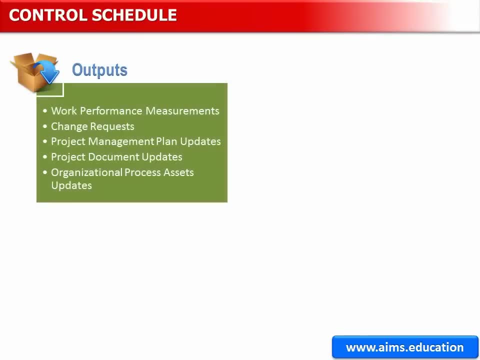 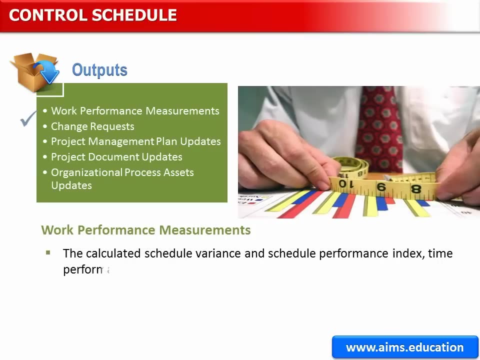 Outputs for control schedule. Outputs for control schedule. Work performance information, The calculated schedule variance and schedule performance index. time performance indicators for WBS components in particular. the work packages and control accounts are documented and communicated to stakeholders. Change requests are processed for review and documentation. 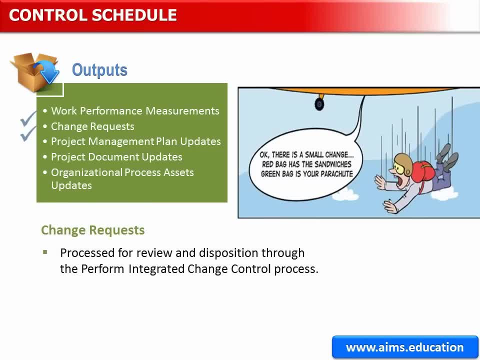 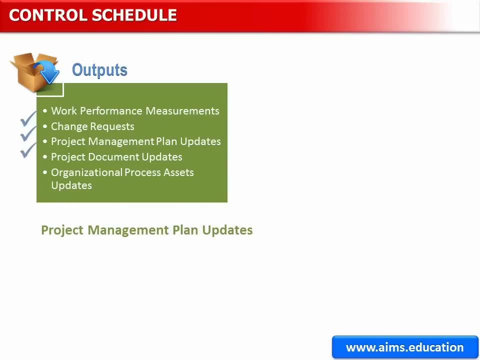 The schedule management software In the next step. This is the highest variable that is set up and is also the current variable that is being used to calculate the entire schedule. In the following slides we will discuss the changes for the WBS components. 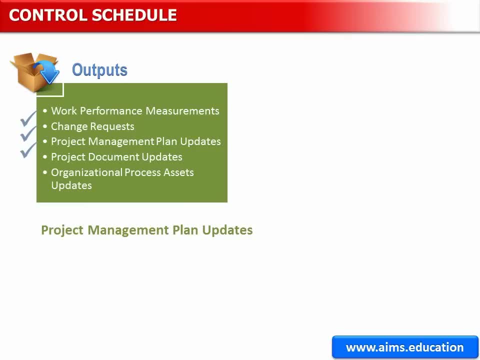 The WBS components are cleaning the schedule number and the time range. The excellence in details are the same as we have done. as an example of such changes, The control control software Baseline may be updated to reflect changes caused by schedule compression techniques. 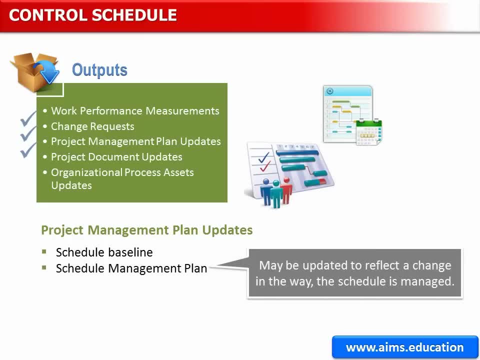 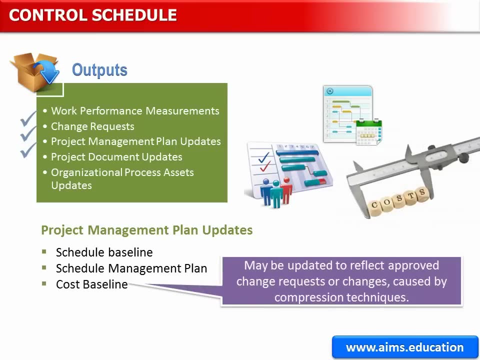 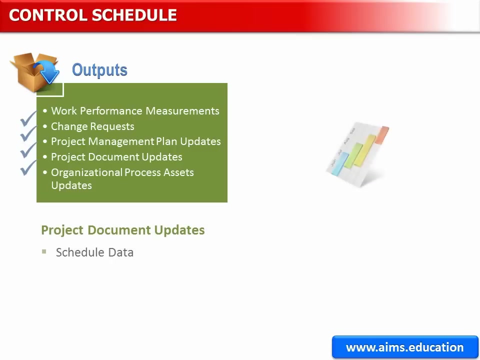 The Schedule Management Plan may be updated to reflect a change in the way the schedule is managed. The Cost Baseline may be updated to reflect approved change requests or changes caused by compression techniques. Document documents that may be updated include, but are not limited to: 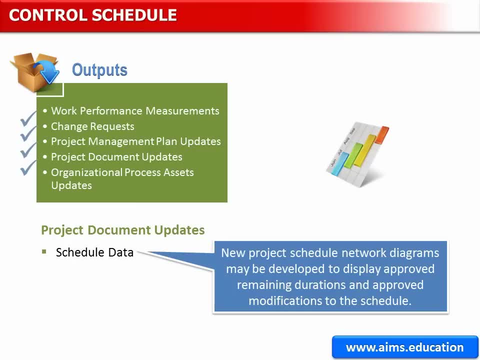 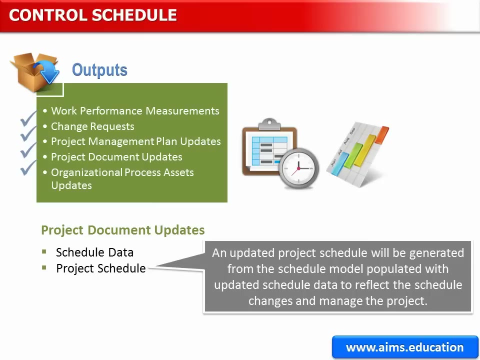 Schedule data. New project schedule network diagrams may be developed to display approved remaining durations and approved modifications to the schedule Project Schedule. An updated project schedule will be generated from the schedule model, populated with updated schedule data to reflect the schedule changes and manage the project. 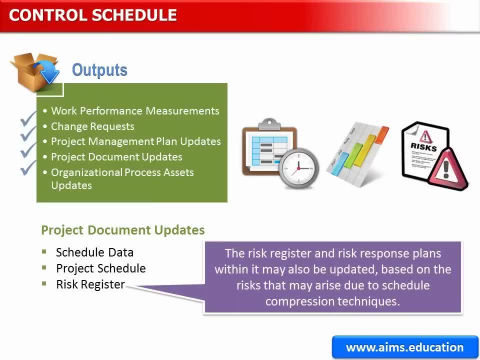 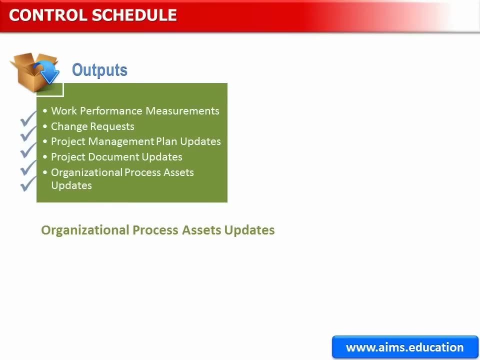 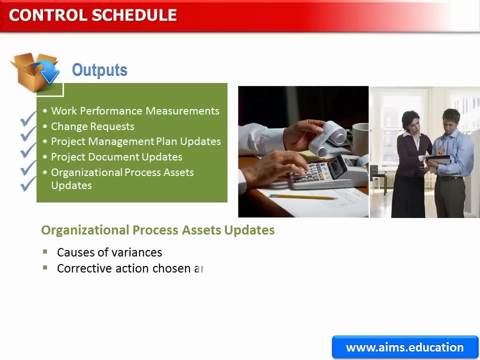 The risk register and risk response plans within it may also be updated based on the risks that may arise due to schedule, compression techniques, Organizational process. assets that may be updated include, but are not limited to, causes of variances, corrective action chosen and the reasons and other types of lessons.